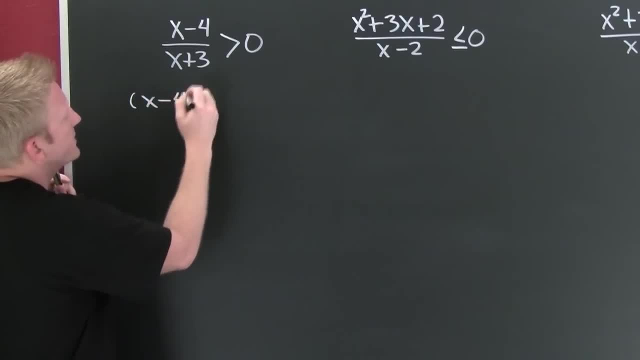 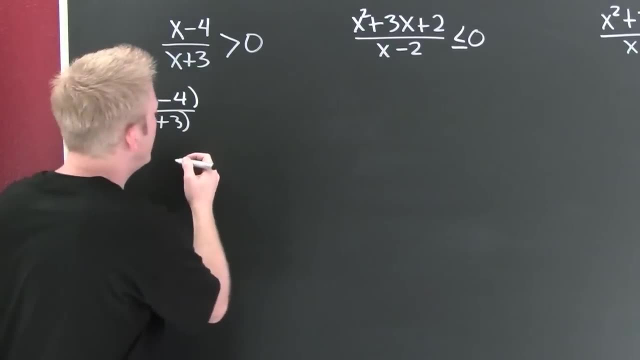 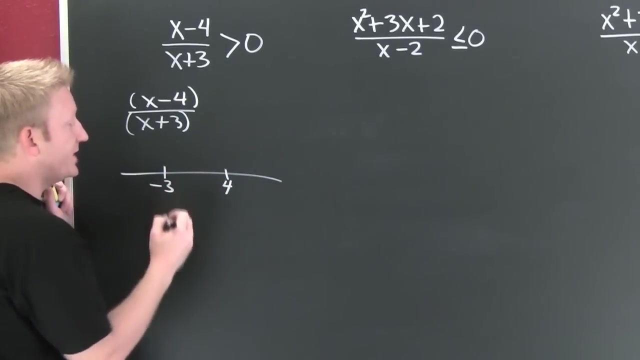 So we factor first. You're like: hold on, guys, X minus four over X plus three. We want to know where the numerator is zero and where the denominator is zero. We find that the numerator is zero at four, Sure, And the denominator is zero at minus three. That's where we got. 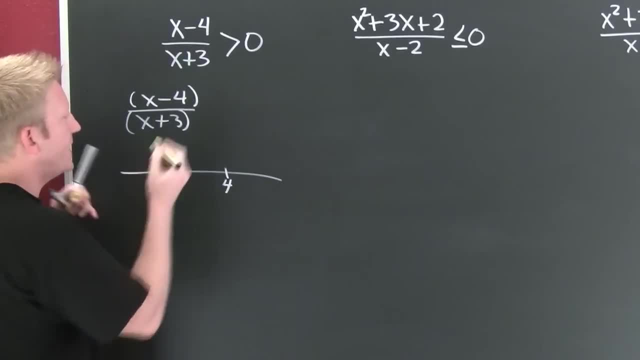 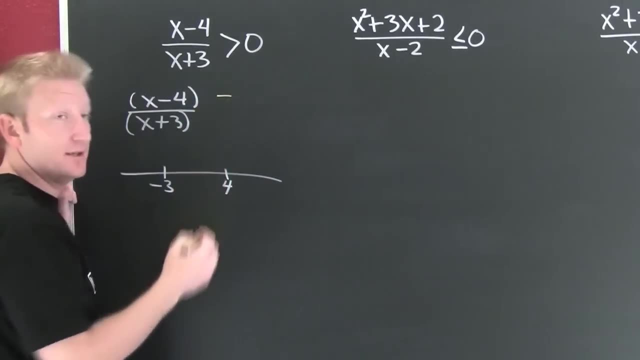 our critical values. Now we need to test some points. I'm looking at the signage of this guy. When I have a number less than minus three, how about minus 10? Minus 10 going to make that minus right. Not real concerned about the signage. Oh, super concerned about the signage, not the. 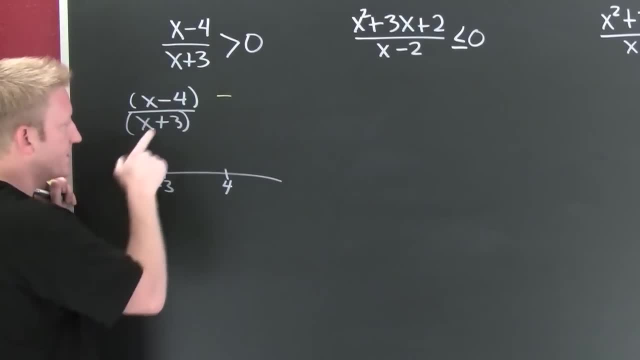 actual retail value of the quotients. Oh, minus 10 is going to make this a minus. Minus over minus is plus. Okay, Check a number in here, In between minus three and four zero's in there. So let me check: zero. Zero's going to make this. minus Zero's going to make this. 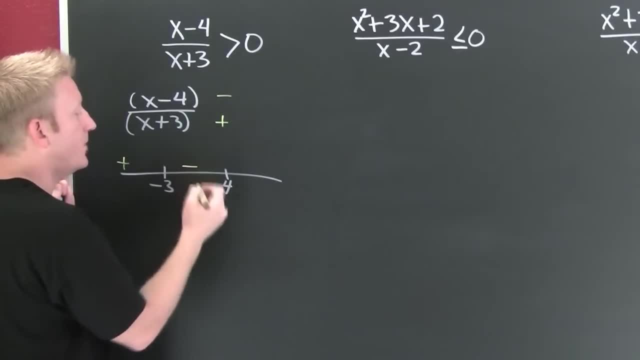 plus A minus divided by a plus is minus. Then I need to take a look at a number bigger than four. Sure, That number would be 10,, 20, or a million, I don't care, just as long as it's bigger than four, because all the numbers that are bigger than four are going to behave. 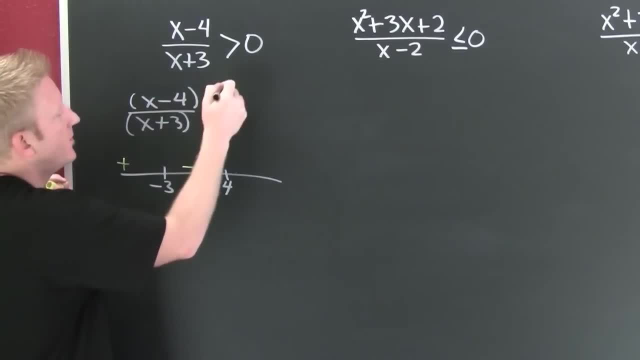 the same way in that quotient. Yeah, So 10 makes this positive. 10 makes this positive Positive. divided by positive Positive, Very nice. Now we need to revisit and look for our solution set. I'm looking for the ones that are bigger than zero. Are those the positive? 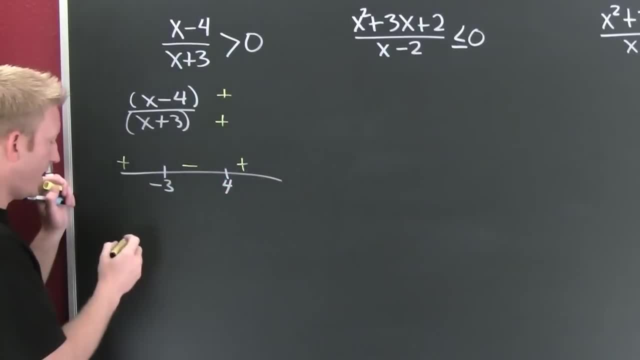 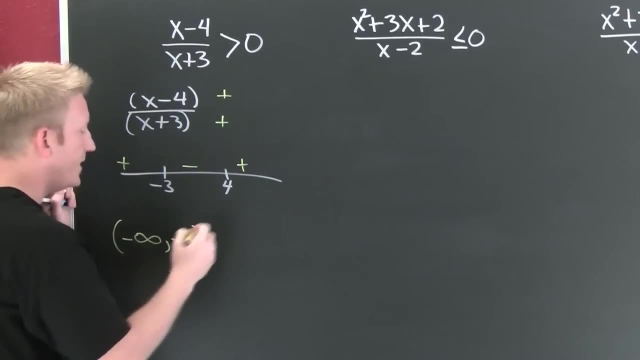 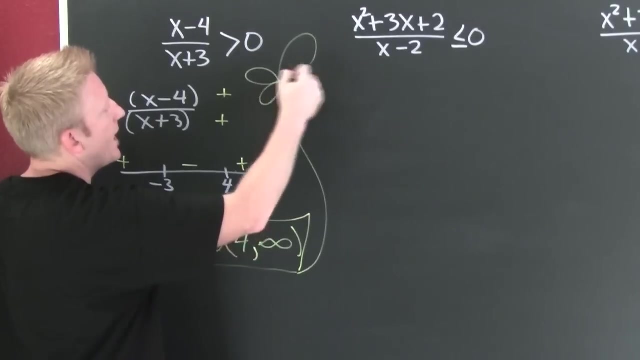 The positive ones or the negative ones? They're the positive ones. Yes, So then that's minus infinity: Two. three to heat included, Don't In onion width. four and a whole lot more to infinity and beyond. A box and a flower, Is that right Now? I'm taking a look at this. 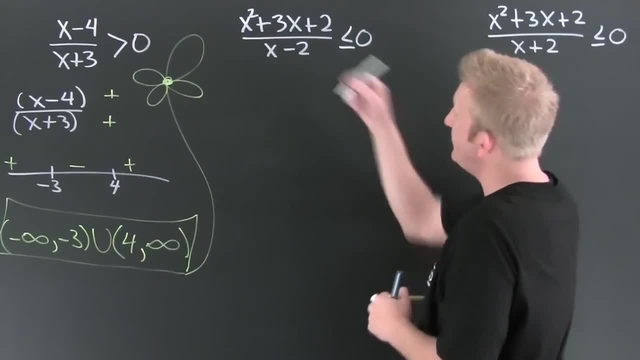 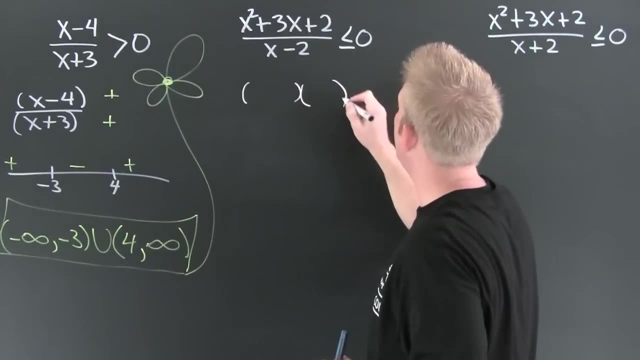 next. Oh, I need to factor first Factors of two that add to be three. Are there any? You got to get that. You got to get that. Two and one, X and X, The signs are the same and they're. 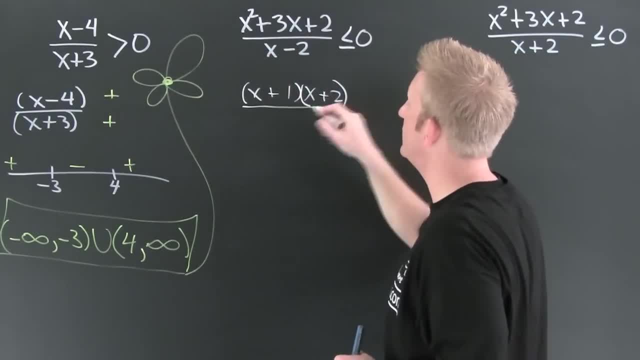 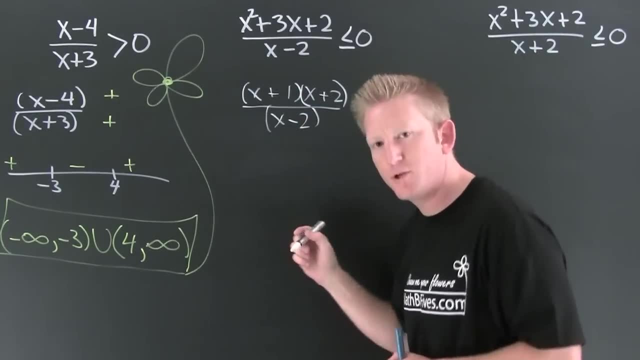 both positive, positive positive All over X minus two. Oh Okay, So then here people, what I'm trying to do is I'm trying to get the zeros- Zeros of the numerator and zeros of the denominator, All right, 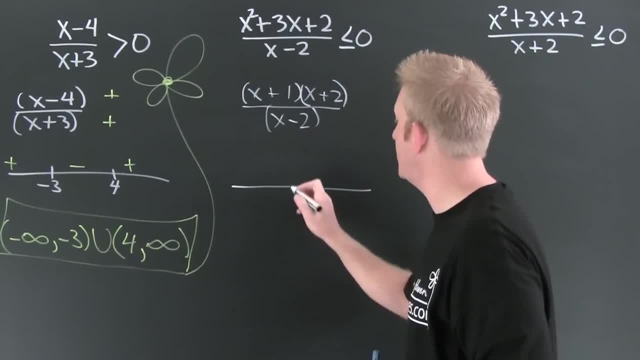 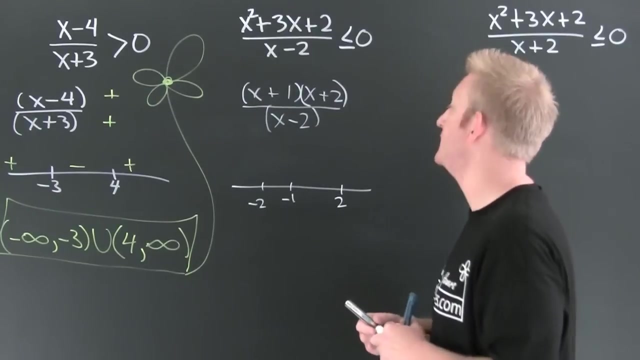 They are all critical values. In my numerator, I see I'm going to have a minus one and a minus two, Ooh. And in the denominator, my critical value is two. Yes, Okay. So now let's take a look at a number less than minus two. A number less than minus two is a minus ten. 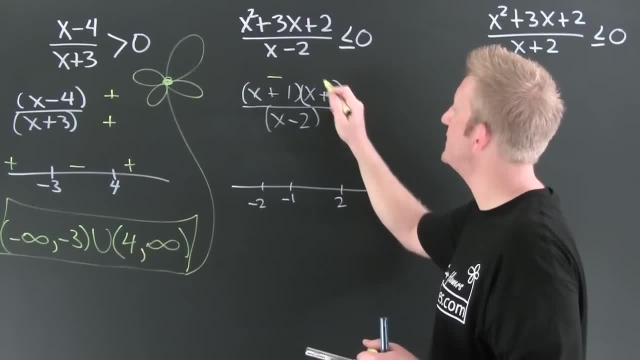 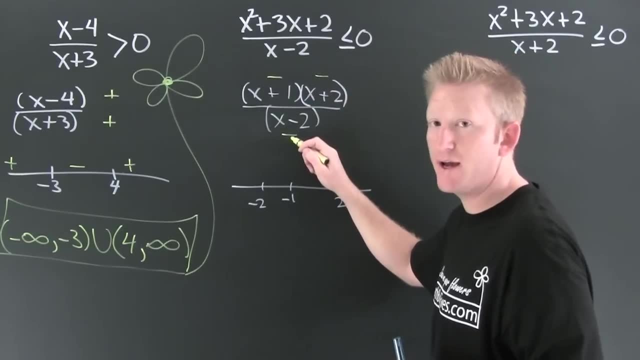 and that makes this negative. A number less than minus two is minus ten, and that makes that negative, And minus ten makes this negative. Negative times negative divided by negative. There I see an odd number of negatives, So my quotient's going to be negative. Now I need to go in. 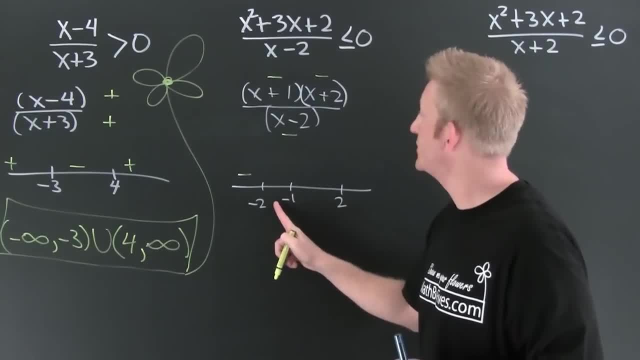 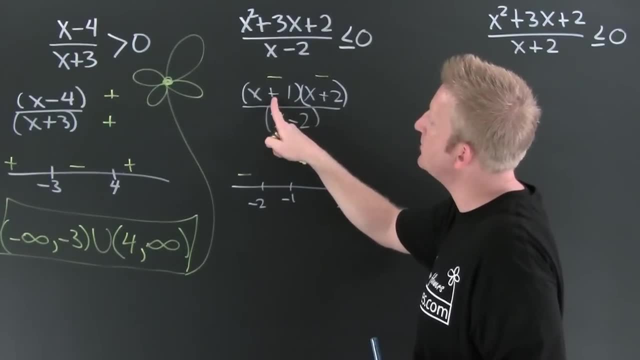 here Minus 1.5.. Okay, That's in there. Sure, Go decimals, Go decimals. Yes, Um, I put a minus 1.5 in here. Yes, Is this going to be positive or negative? It's going to be negative. 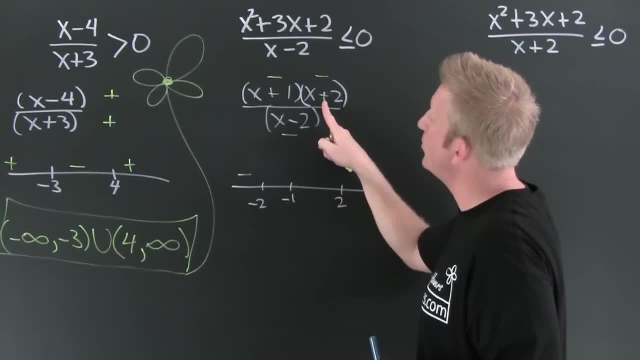 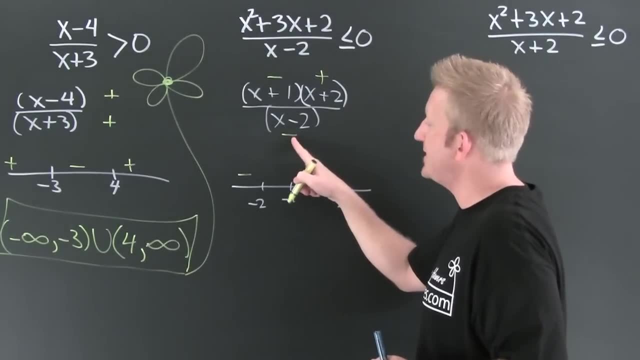 because 1.5 is bigger than one. So I put a minus 1.5 in here and the two overpowers him, making that plus. I put a minus 1.5 down here and that's negative. So this is going to be. 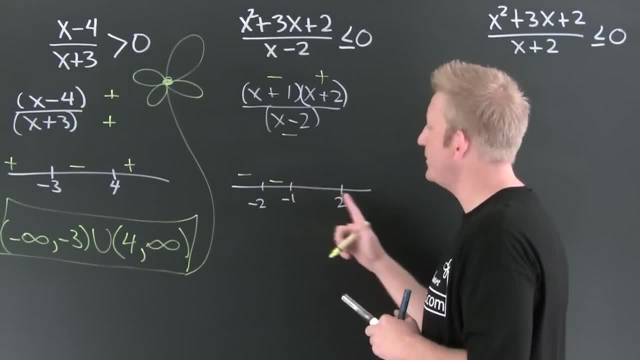 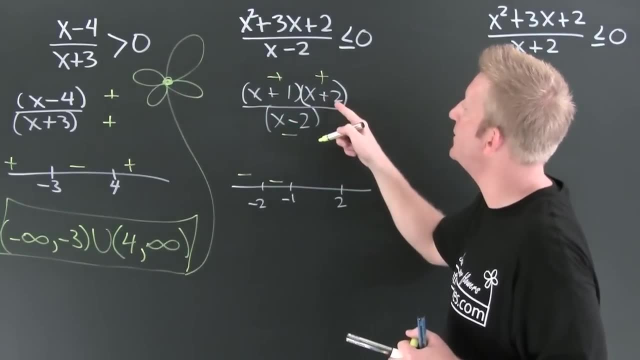 negative. Very nice, I keep on keeping on All the way to a number in between minus one and two. How about zero? So I put zero in here. That makes that factor positive. Zero in here positive, Zero in here negative. Positive: positive divided by negative, negative. 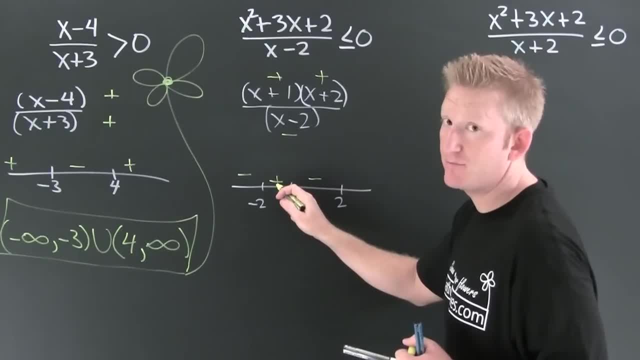 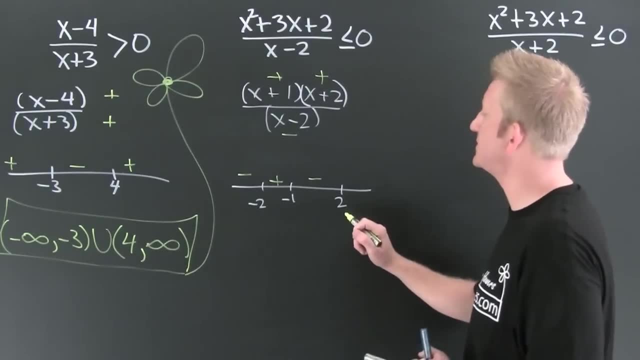 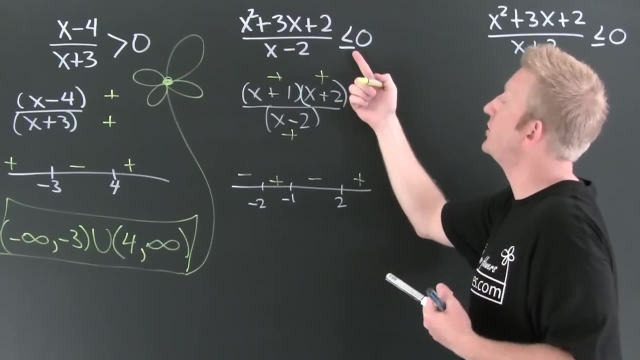 Whoa, Back that step up. That one was positive, wasn't it? Yes, Now I'm on a number bigger than two. Oh Yes, Ten. Positive, positive, positive, positive. Now, what am I looking for? I'm looking for. 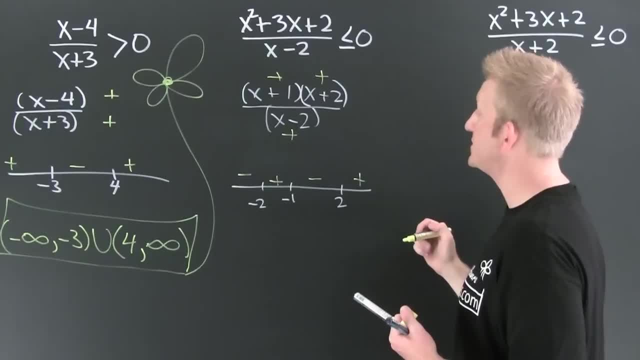 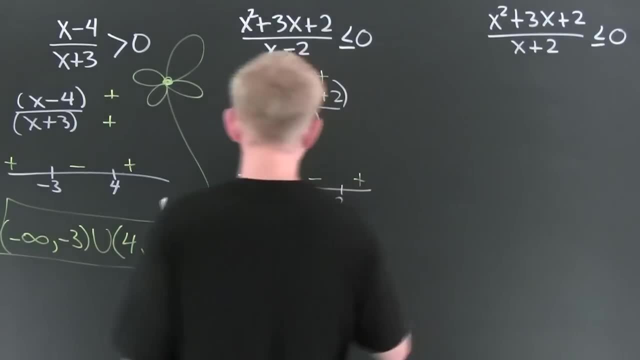 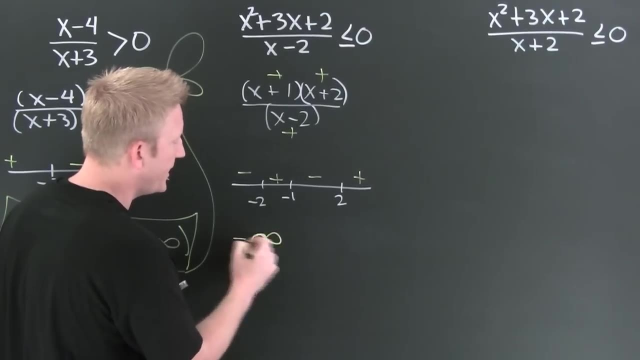 where this is smaller than zero, Sure, Where is it smaller than zero? It's smaller than zero here, and it's smaller than zero in here. Okay, So then here we go. I need to go all the way from minus infinity, Yes, To minus two, Oh. 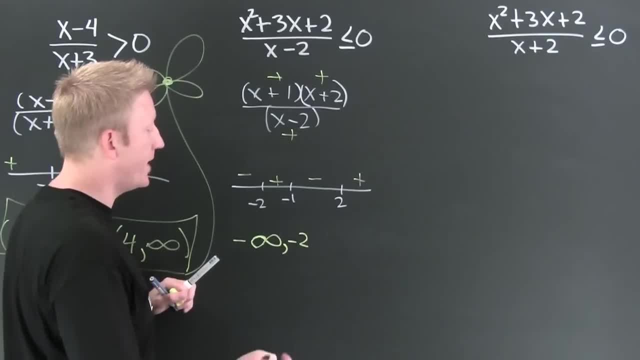 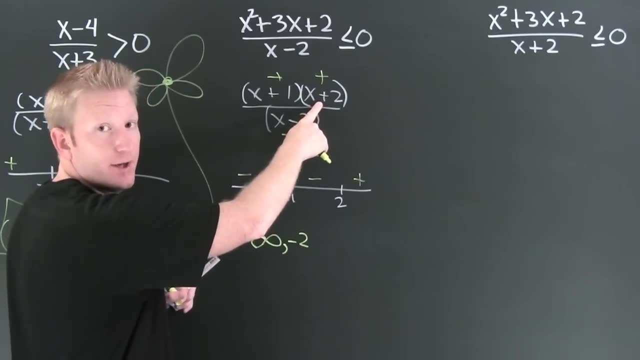 Well, oh, now we need to see if we can include a minus two. The minus two is going to make that one zero. Zeros in the numerator are fine. Had it made a zero in the denominator, oh, We couldn't include that, Okay, Because, um, you can never divide by zero. Anyway. 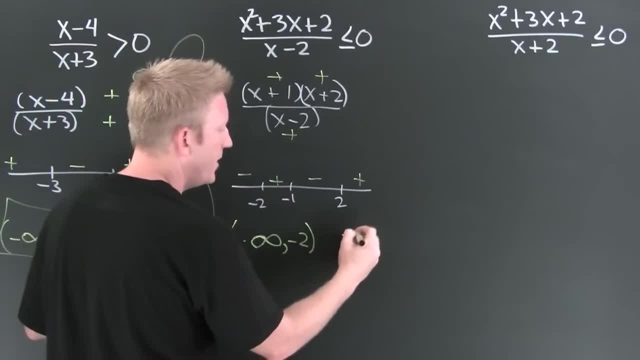 that being said, close it Also from minus one to two. Oh, can I include minus one? Uh, I'll just have to. Yeah, Okay, okay, Ann, treaty will definitely not make it our case, but if you do repeat the values, I'd like to see you all roll out with another test score for. 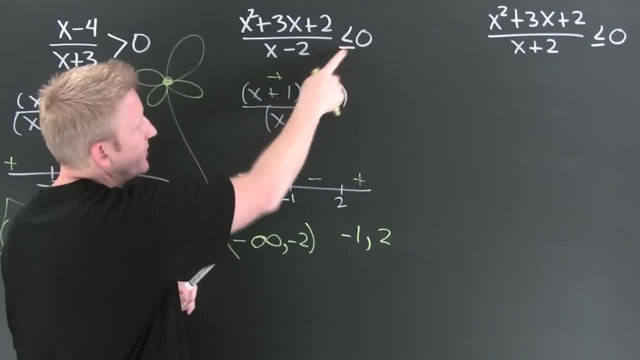 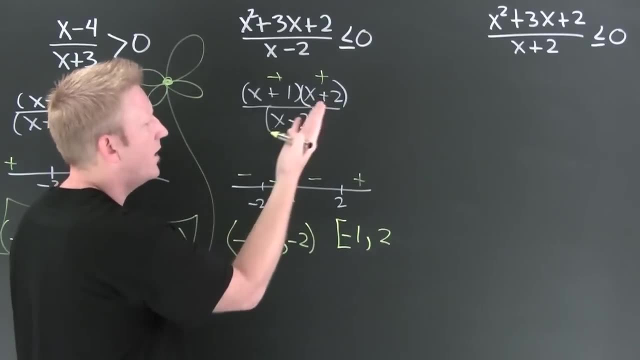 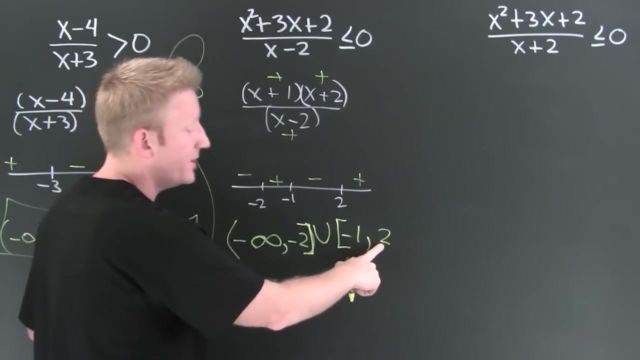 I can. yes, because I'm looking for the or equals to can include minus one. hey, was I including two? yeah, all right, Ken, you're messing up here. you go that one's good onion, that up with minus one. okay, so now here's the sticky spot. we know. 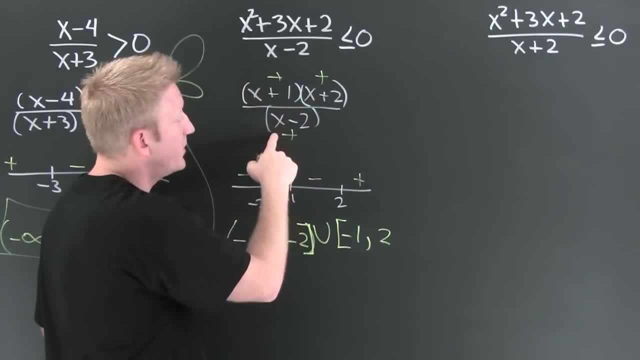 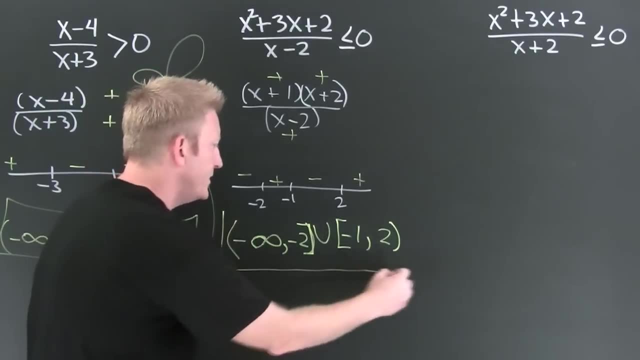 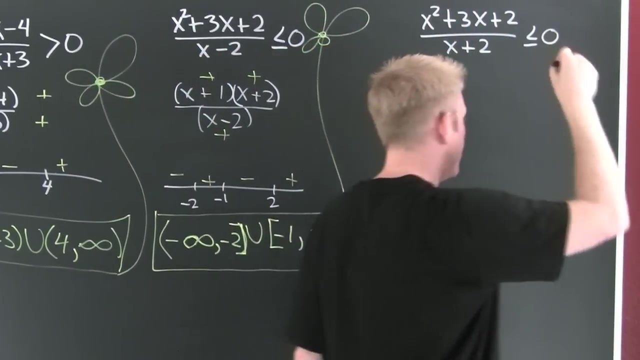 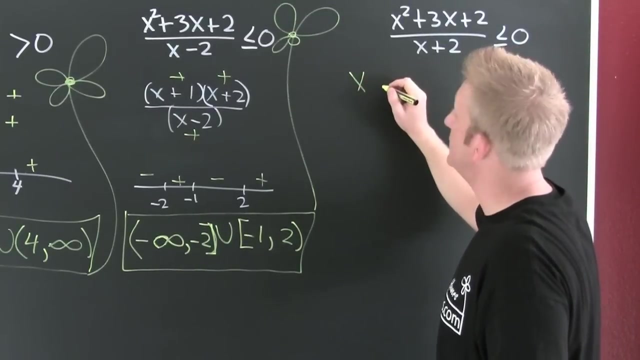 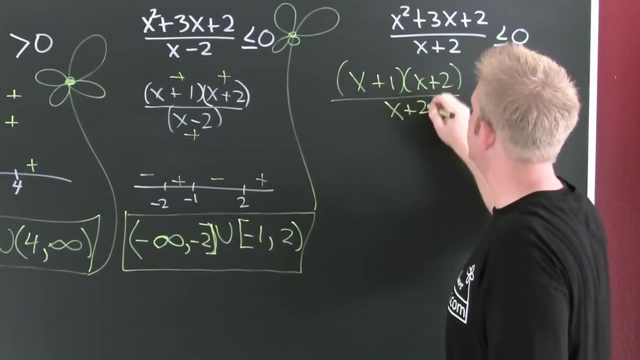 we're including the endpoints unless there's zeros of the denominator. this one is a zero, the denominator, so you are not included. okay, on the one that's real similar to my last example. why? because, in fact, is real similar. but hey wait, there's more factor. first, X plus one, X plus two over X plus two. you know what? 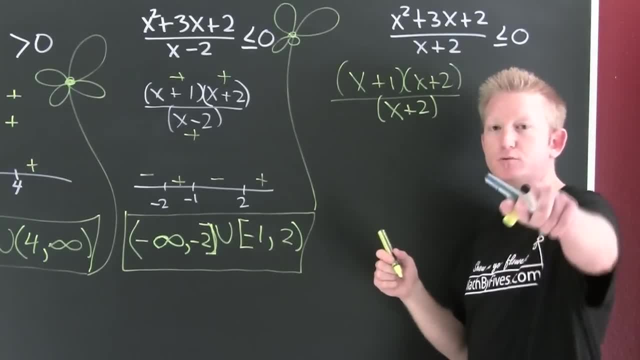 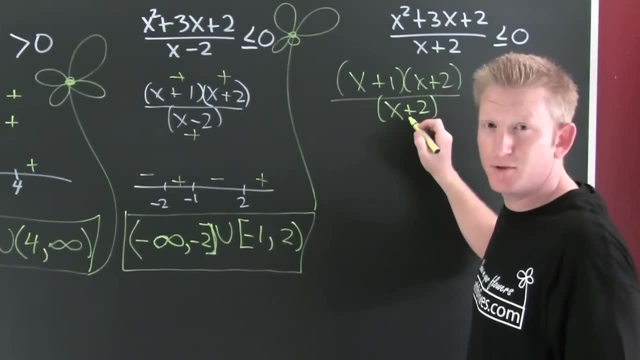 are you trying to do? you know what are you trying to do. you know what are you trying to do. you really want to reduce those, don't you? don't you even try it right cuz let's see what happens. this is um a possible domain restriction because you 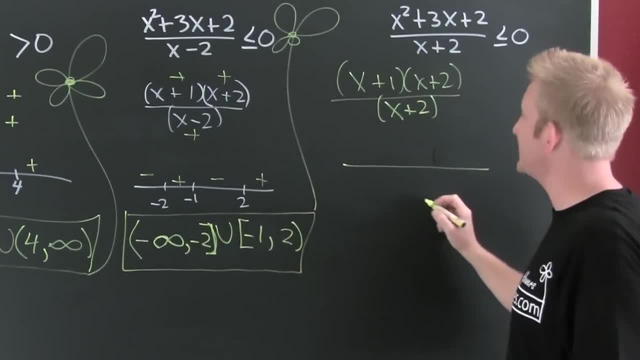 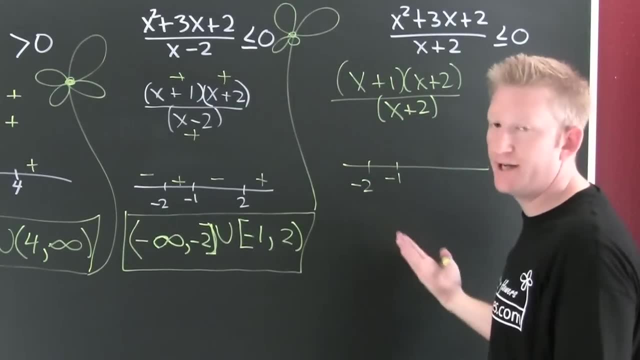 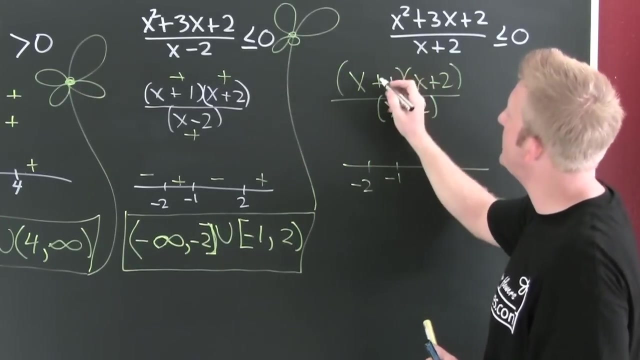 can never divide by zero. yeah, so then I put my critical values on the number line. here I only see minus one and minus two. oh, probably could have planned that better. all right, so now I'm up here. yes, a number left of minus two. how about minus ten? minus ten makes 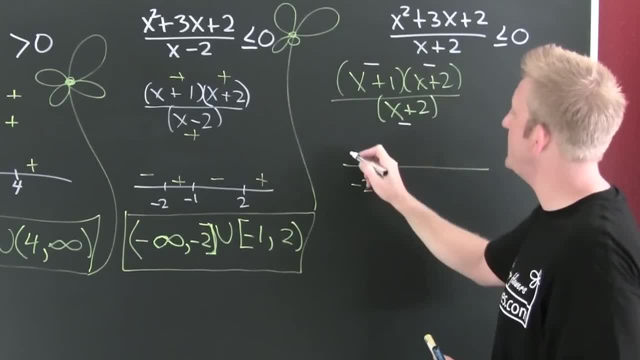 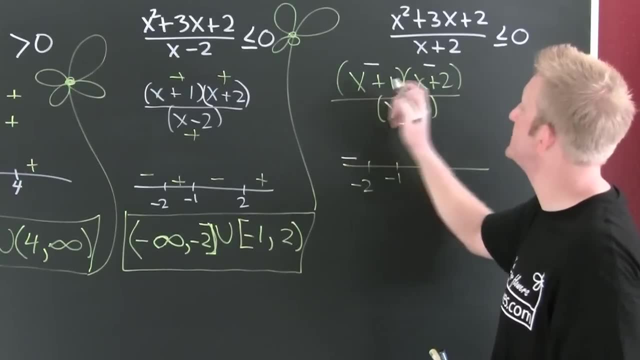 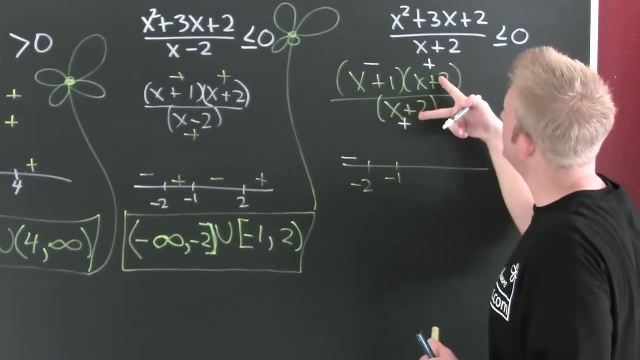 this minus minus and minus three minuses make minus. yes, in between here, 1.5 minus 1.5 makes this minus, makes this plus, makes this plus. it's changing both those signs at the same time. huh, okay, sure, and the whole dang thing is gonna be minus. 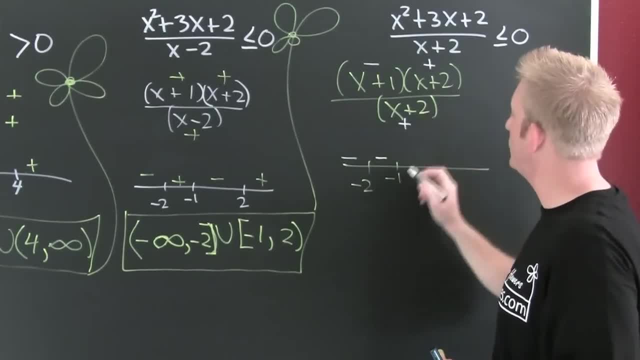 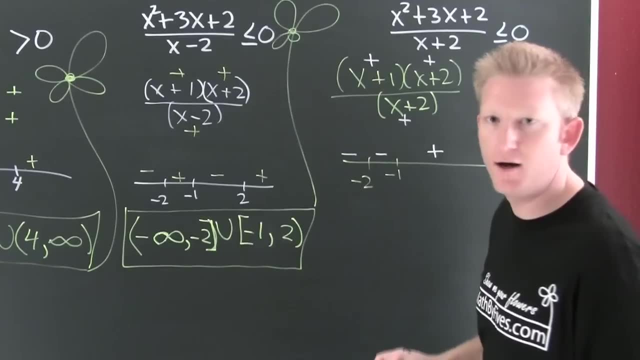 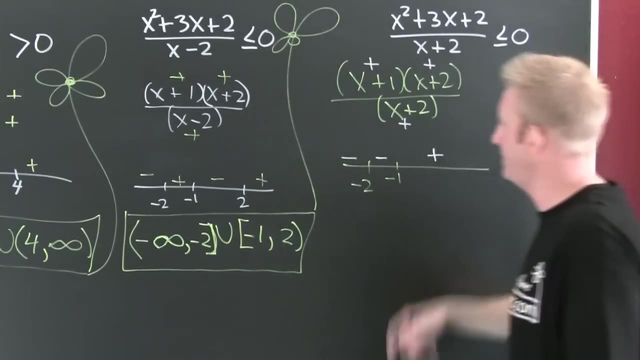 yes, but wait, there's more. what about a number bigger than minus 1? 0? 0 makes this plus plus, plus plus over here, uh-huh. so now we need to concern ourselves with the solution sets. we want the negative ones that are smaller than 0, mm-hmm. okay, so then here. 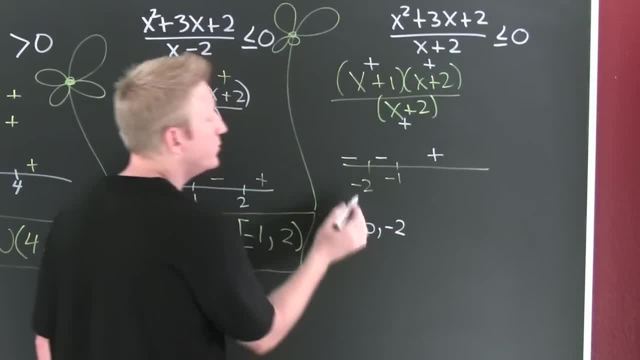 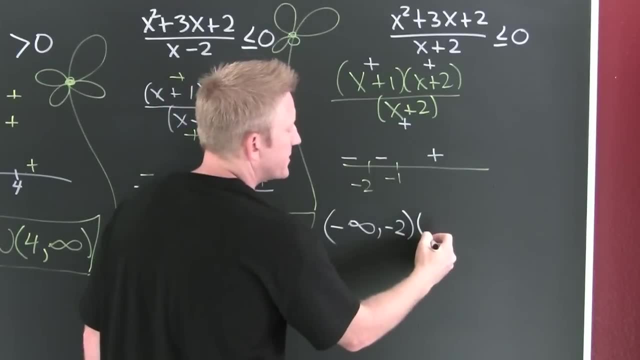 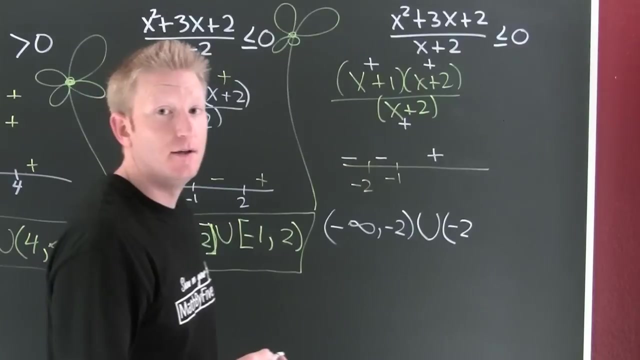 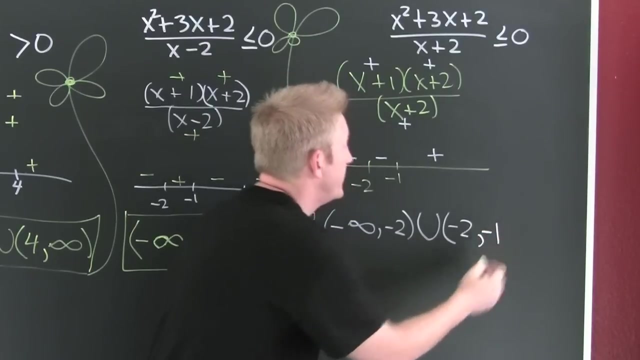 this goes from minus infinity to minus 2. oh, why can't I include minus 2? because it makes the denominator 0 right and this act of leaving out minus 2 is written like this in interval notation. so now I also need to go to 1, all the way to minus 1. do I get to include minus 1? 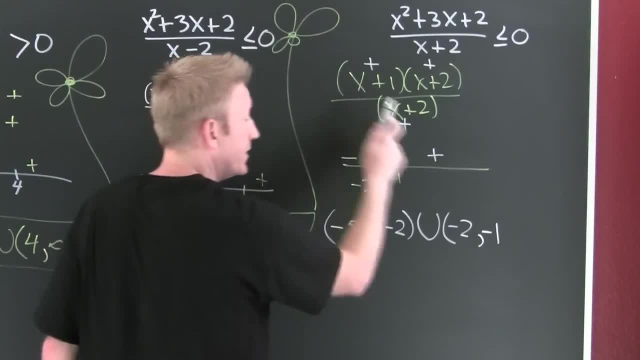 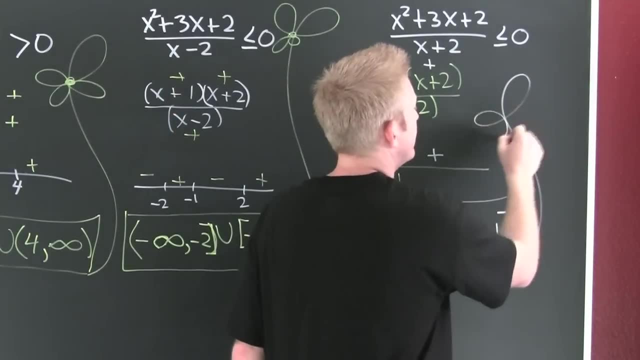 because it's the or equal to, and it's a 0, the numerator I do, and a flower. 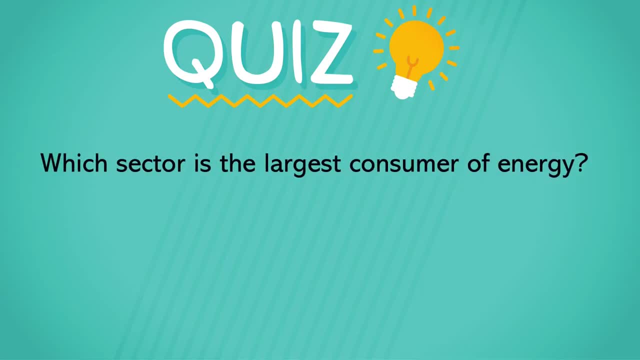 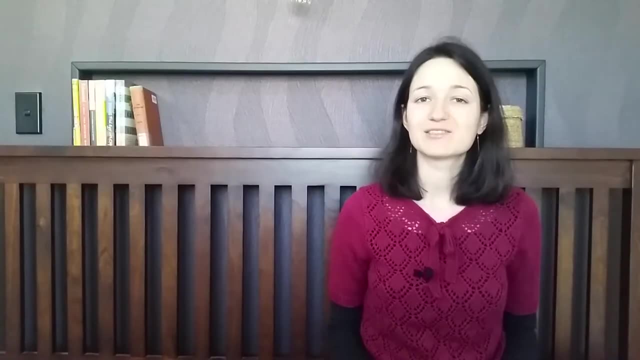 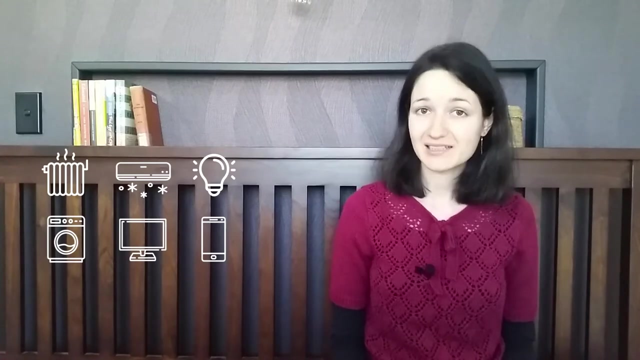 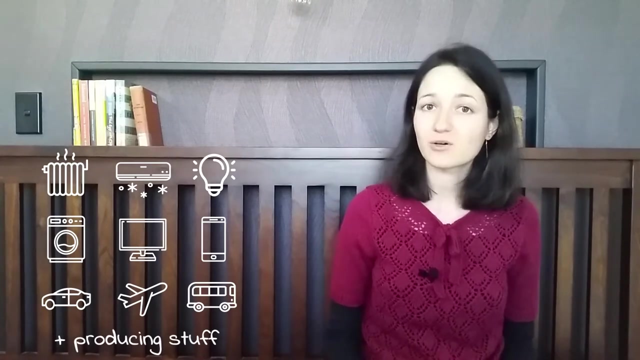 Energy is ubiquitous in our lives. We use it to heat and light up our homes, to power the various appliances and gadgets that we have to get places. it is used to produce everything we buy. But all this comes at a huge cost to the environment and subsequently. 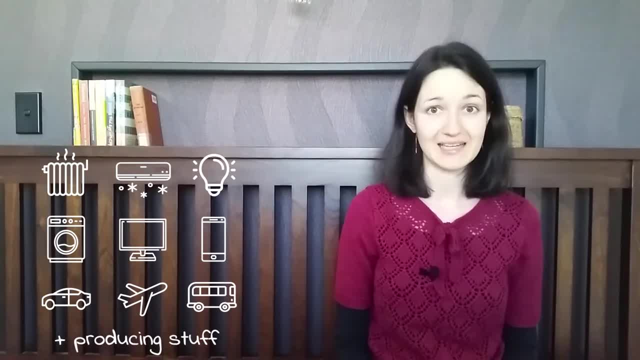 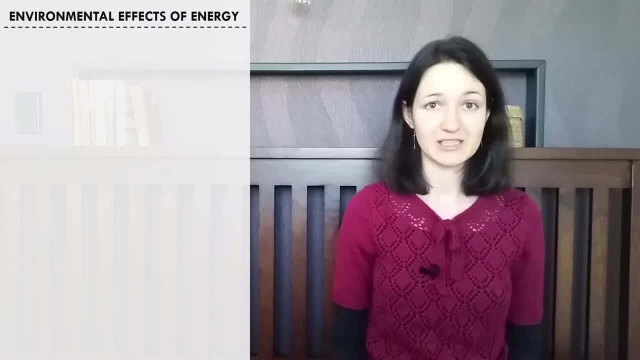 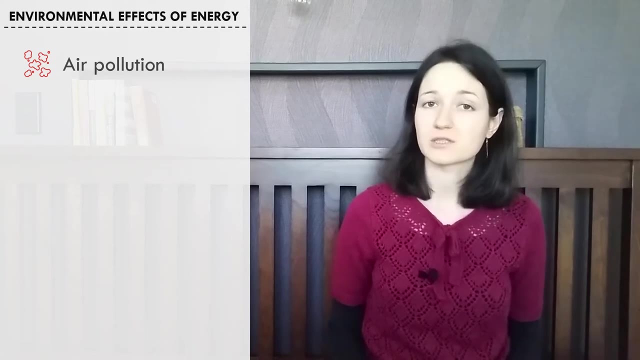 our own well-being. What exactly the problem is and how to reduce it is what this video is about. Let's do this. One of the biggest issues with energy is air pollution, and air pollution is very harmful to human health. It is estimated that air pollution is responsible for 5 million. 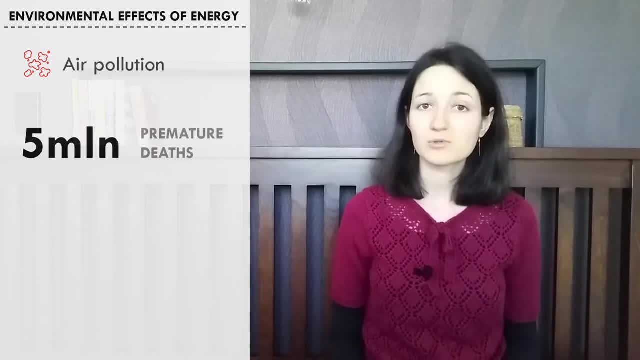 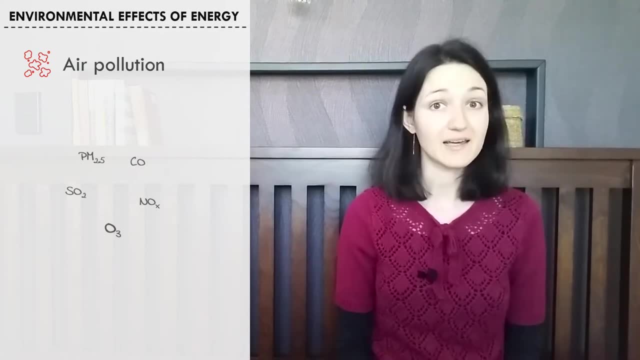 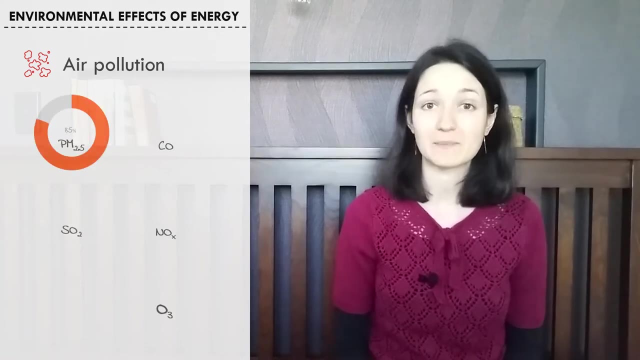 premature deaths globally every year, which is almost 1 in every 10 premature deaths. There are 5 major pollutants that are responsible for these deaths, and energy is the single biggest source of each of them. It accounts for 85% of particulate matter.